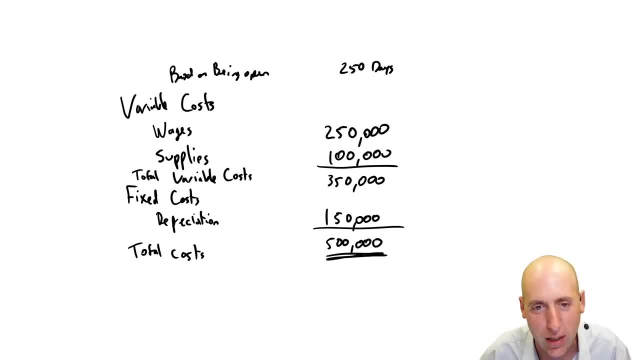 doesn't come till later. great. more golf days or less golf days are going to depend on when frost sets in on the golf course And it turned out the season he was talking about. So this is the budget: 250 days, the actual season. they golf 300 days. it was just a warmer than usual season, The only a couple months where it was under snow and ice and it was frozen. but they actually were open 300 days And, as a consequence, you know they had 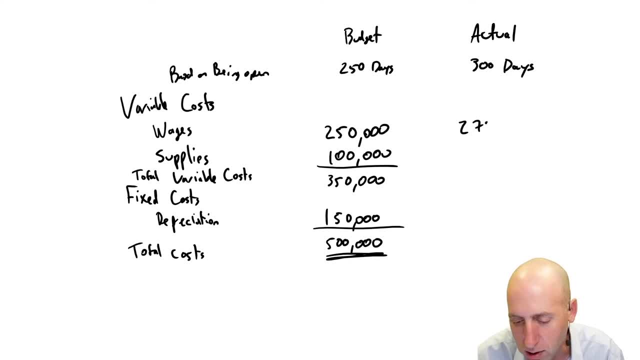 different results from what they budgeted. they spent $275,000 on wages. they spent $110,000 on supplies. that was $385,000. And their equipment depreciation was $148,000.. For whatever reason, maybe they got rid of a piece of equipment or something like this. So the overall cost actually let's make it 145.. So it's an even number here. Let's see five and five. 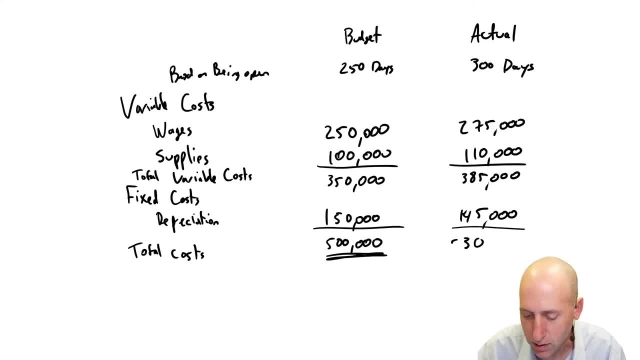 was three zero $530,000. So their overall cost for 530.. And the thing that happened to my friend was kind of a shame. The boss came in and gave him a hard time. They said: Look at these variances. You were off 250 to 275.. You blew the budget by 25,000. is 25,000 unfavorable? You blew your budget here by 10,000 unfavorable. The only place where 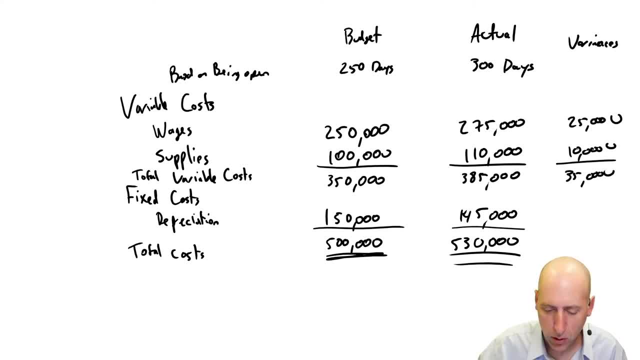 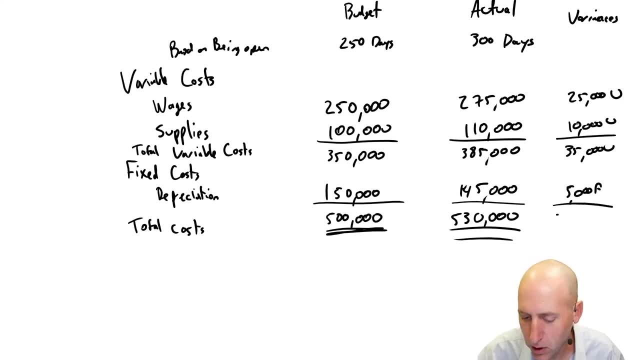 this is 35 unfavorable. The only place you made your budget was the place you didn't have a lot of control over depreciation. you are 5000 favorable, but overall you are $30,000 to the bad. you did a bad job here, friend. What do you have to say for yourself? And I hope you're looking at this and saying, Yeah, he did go over budget, But this is not justice And the reason is they were open. 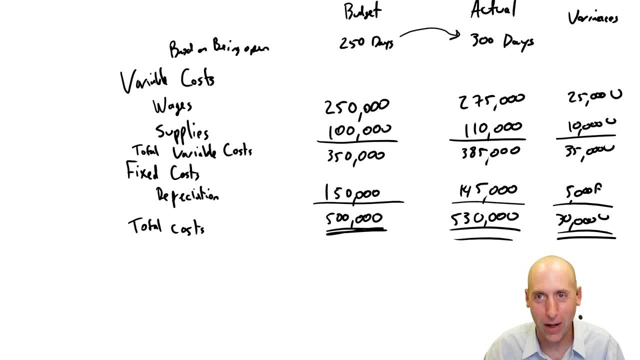 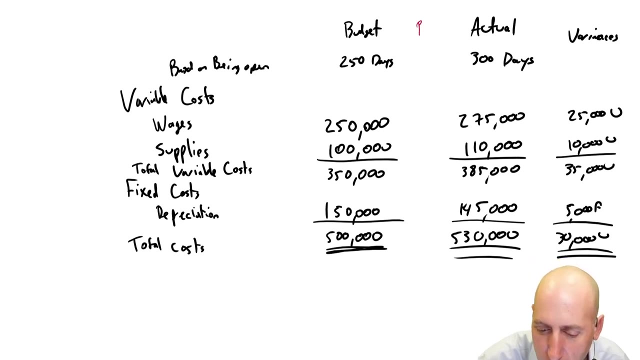 so many more days, we would expect them to go over budget And what we should do is not compare them to their static plan, their plan of 250 days. we should say, Okay, let's pretend, let's go back in time, let's give ourselves a time machine. If we could redo the budget as a flexible budget, what would we say if I could go back in time and tell my previous self: hey self, let's make a flexible budget. 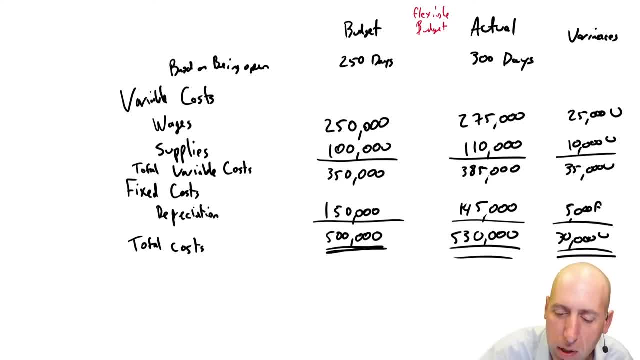 As if we knew that we would be open 300 days. what would I budget for? And the truth is I wouldn't budget for 250 or 100 in wages or supplies. they're variable costs. they vary with the amount of days open and the amount of days worked. So I got to make a new budget based on this flexible data And let's see what we do. So I ignore the actuals, I don't even look at the actuals, I just pretend I didn't know. 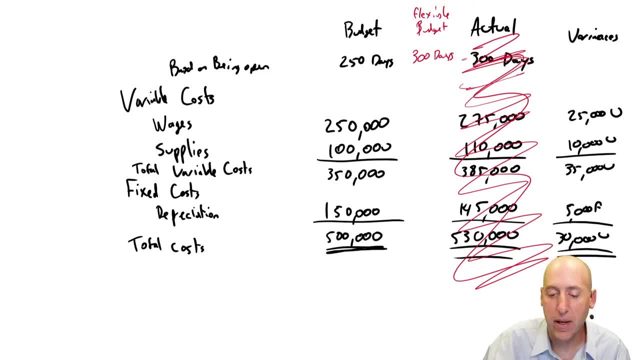 that and I make a new budget based on 300 days. so my wages were $250,000 based on 250 days. well, what would they be? based on 300 days, they'd be three hundred thousand thousand dollars a day. my wages would be three hundred thousand. 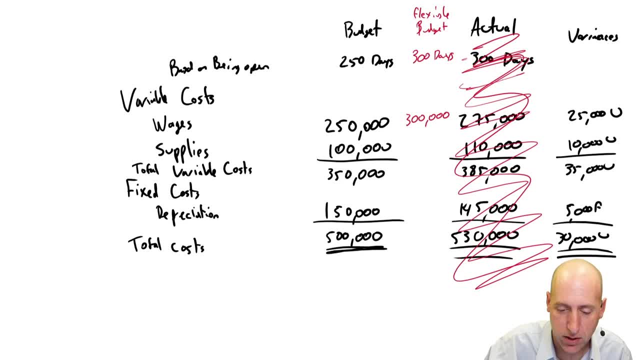 dollars. my supplies? a hundred thousand dollars based on 250 days. what would that be? I got to open a calculator figure out what that would be. I have no idea if it was a hundred, not one, nine, nine. oh, my goodness, my calculator is getting away from me. a hundred thousand dollars based on 250 days, that's four. 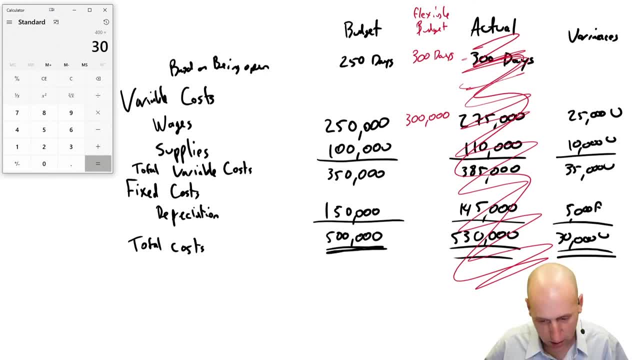 hundred dollars a day. well, four hundred dollars a day for 300 days is a hundred and twenty thousand dollars. 300 plus 120 is 420. now again, before the year I didn't know, I sold this equipment, so I would have just budgeted depreciation to be 150 and if, knowing what I know now, I would have given my 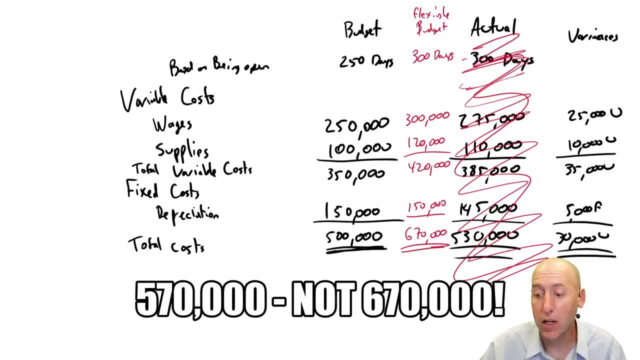 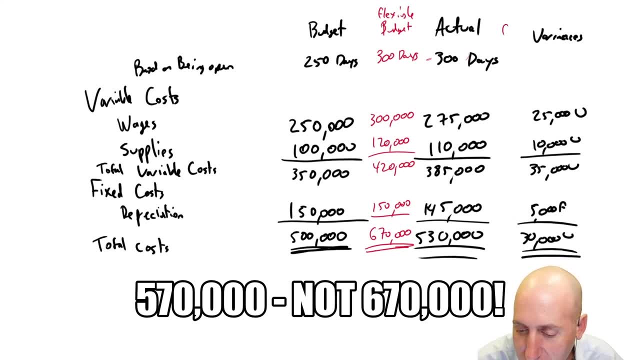 friend a six hundred and seventy thousand dollar budget line. so let's compare that flexible budget to the actual to get a flexible variance: 300 versus 275. twenty five thousand dollars favorable. right he had to. he spent 275, given what we know we would have expected him to.